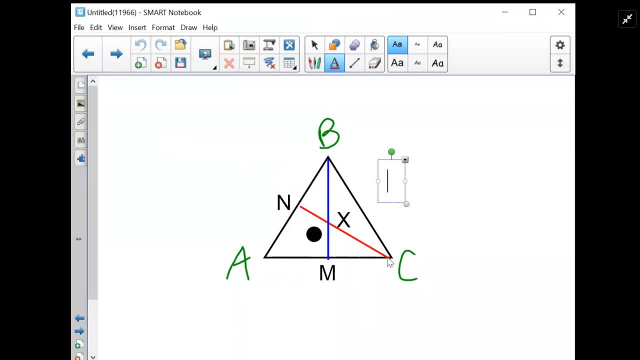 So it bisects ACB, Um, and it goes from C to N, um, and N would be the midpoint here, Anyways, and then those intersect at a point. we're going to call X, because that's what it says. 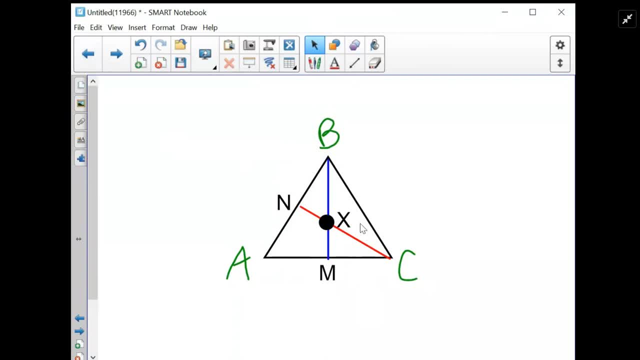 So I'm going to put this little point right here to show that's where it intersects and that's called X. And then they told us it's equilateral and each side is two. So that means all of these are two And that also means 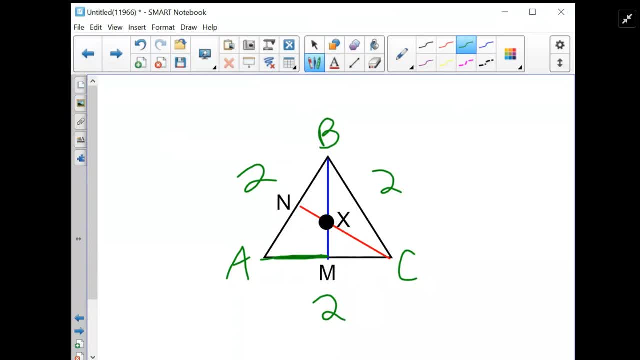 We know a M is one because that's half of two. M is the midpoint which divides the line in half, And then, over here also, MC is one. Okay, So I'm not sure if there were um formulas around to shorten this, but basically what I did, um to get these formulas that I actually found online, but I think they. 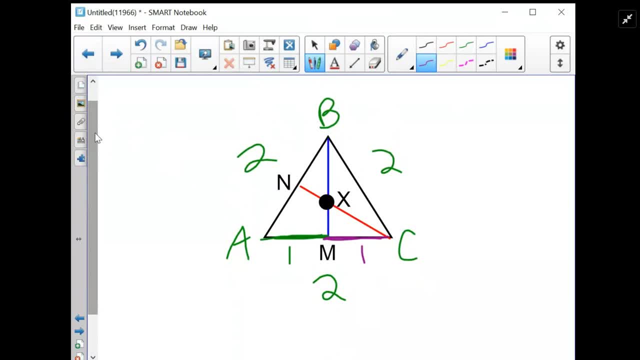 Did the same thing I did is use Pythagorean theorem now to figure out what BM is, because you know this side, you know this side, you know this is a right triangle, Um, and then you can figure out what BX is, once you know what BM is. 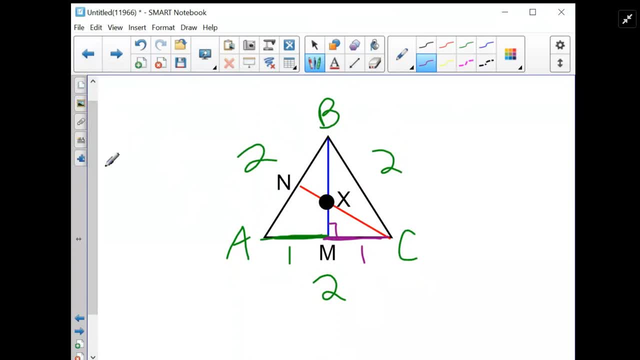 Okay, So using Pythagorean theorem that says that a squared Plus B squared equals C squared. Now remember, C is the hypotenuse, the side opposite of the right angle. So that's going to be your two, and then A and B are just your two straight sides in a right triangle. 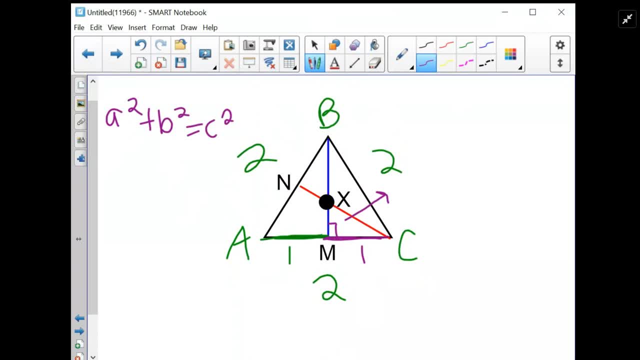 So we'll say that we'll say X or any variable. Don't get confused about X. Let's say maybe Y, um, cause we don't know what BM is. if we need to, We could rewrite it. We could rewrite this triangle like this: 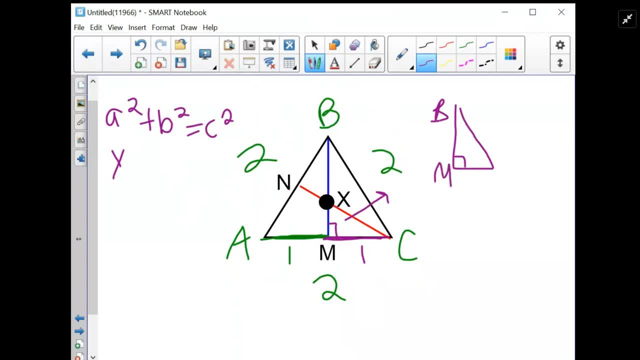 Here's BM and C and we know this is one, This is two, This is, we'll say, Y. That's what we're solving for. So Y squared plus B squared is one squared, B is one and C squared is two squared. 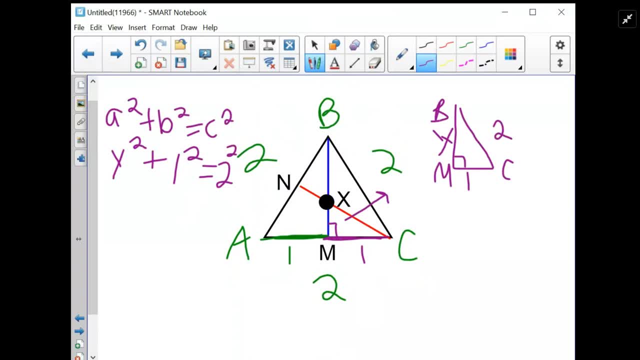 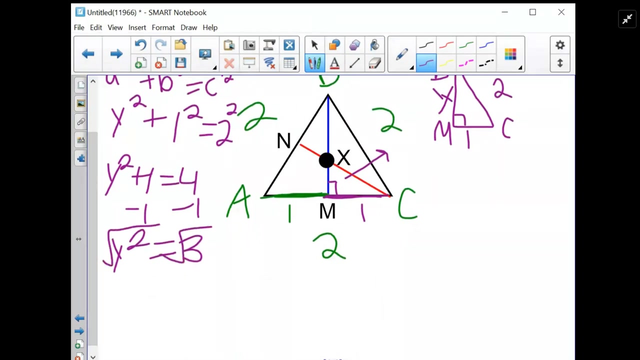 Okay, Um, Y squared plus one equals four. We're simplifying. Then we subtract: Y squared equals three, So our Y here is square root of three. Okay, So square root of three is three. Square root of three is the value of that whole side, BM. 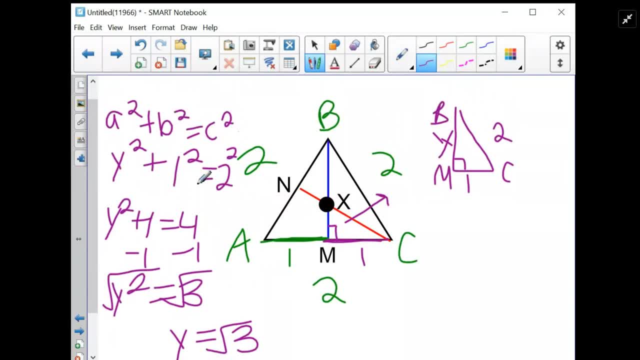 Now here's something else interesting. So that whole side is square root of three, and then the equilateral triangle, your centroid, which is what we're going to call this X, where your uh median and your uh. well, this is also a median cause. all the medians are also angle bisectors. 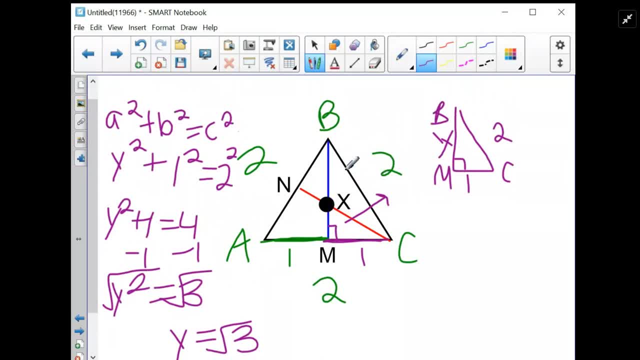 um, where all the medians intersect is your centroid. So what's intersect is your centroid. here It's a ratio of two to one. So this side, from the centroid to the vertex, is two, compared to here, from the centroid to your midpoint, is one. 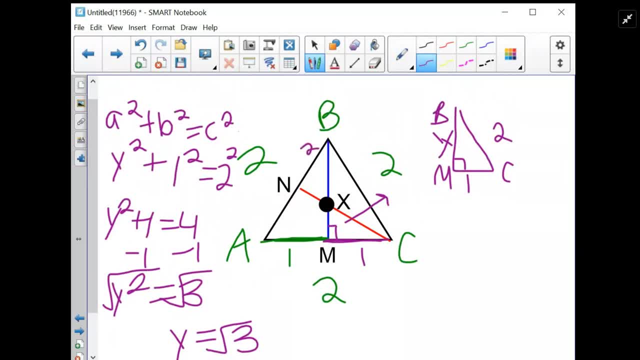 which means this side is two thirds times your length, which we'll say we found was Y, And this is only one third. If it's, if the ratio is two to one, that means two plus one is three is the say that's total length. 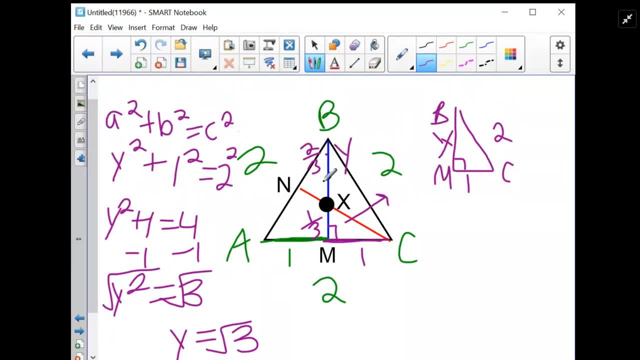 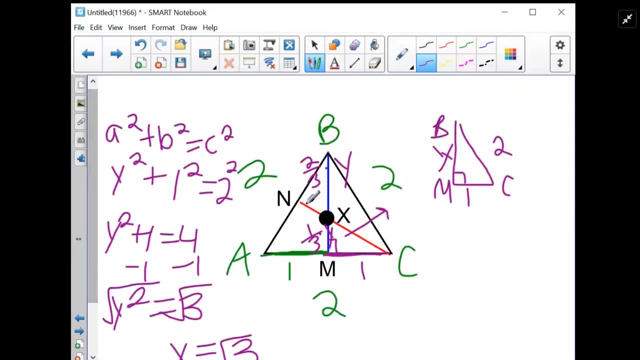 Um, and so if this is twice as long, that's two times um. one third is two thirds and one third anyways. So multiply it times one. So if our Y here is square root of three and we want to find from our centroid to our vertex, 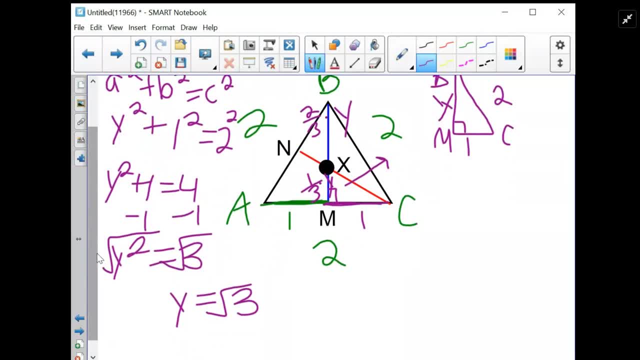 we are going to do, um, square root of three. We'll say over one times two thirds, And our final answer here should be two square roots of three, all over three, And then we could also confirm So um, let me show you. 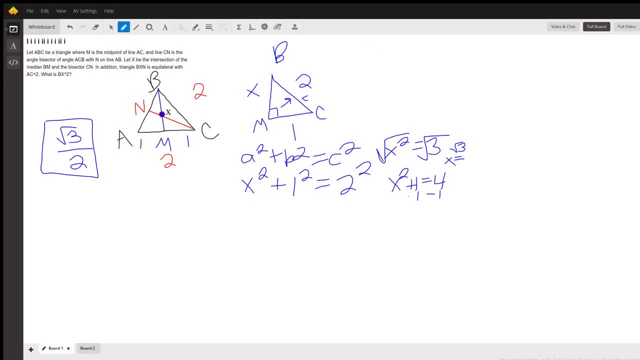 Oh, I'd like to show you real quick My whole screen application window. Oh, you know what? Nevermind, Just. 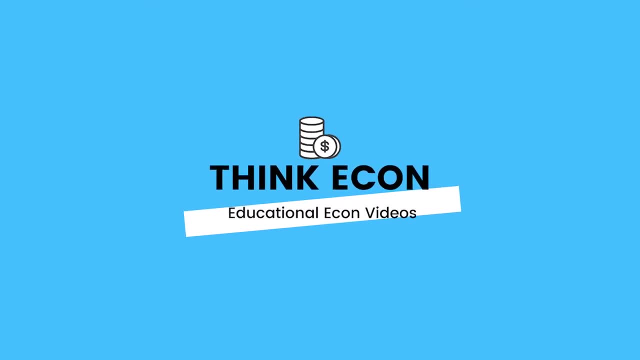 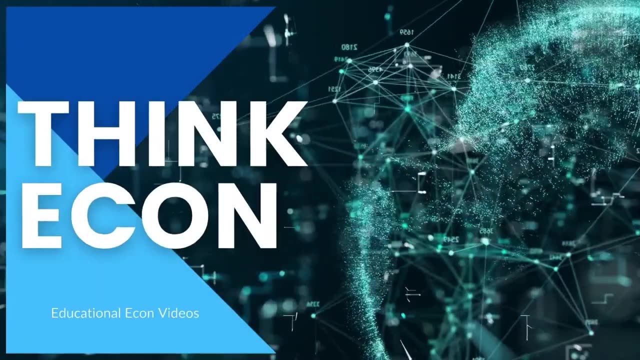 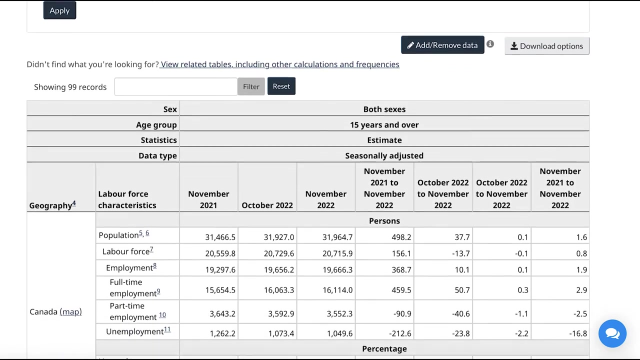 Hey everyone, and welcome back to the channel. In this video, we'll be learning how to calculate the labor force participation rate, the unemployment and the employment rate. With that said, let's get into it. What better data to use than the actual data from the labor force survey collected by Statistics? 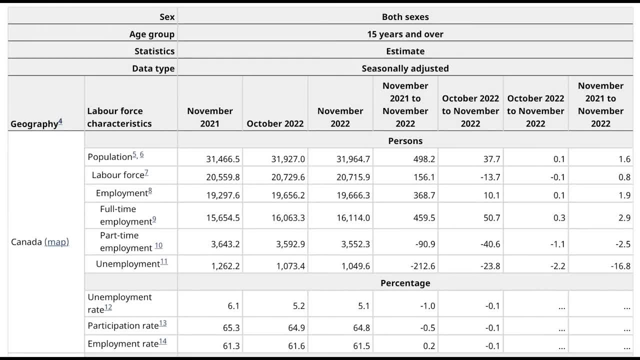 Canada and released to us December 2nd 2022.. So the key information that we're looking at is the population, labor force, employment and unemployment rows. We want the most recent data, so we're looking at November of 2022, as these are the official numbers for Canada. 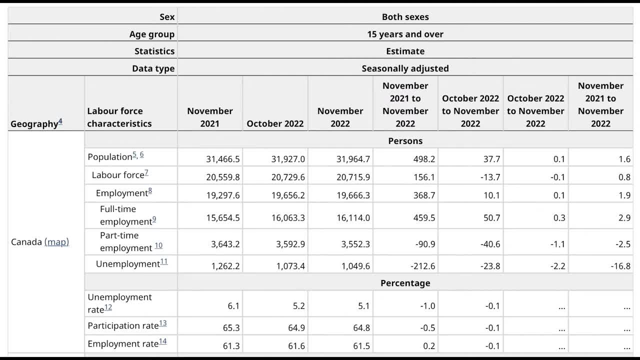 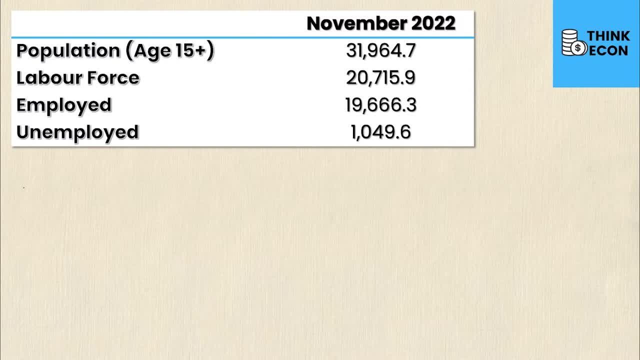 So let's take the data that we want to use and then calculate these key pieces of information. So now I've collected all my data for November of 2022.. Now the population it's worth noting is the population age 15 plus. This is known as the working age population in Canada. 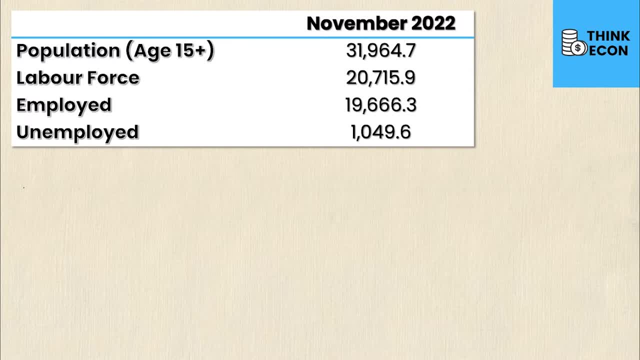 The labor force is the sum of all employed and unemployed people. Now you'll notice, all of these numbers are in terms of thousands. If you took these numbers and multiplied them all by 1000, that would give you the actual. So no, the working age population of Canada is not 31,964.7, but rather 31.96 million. 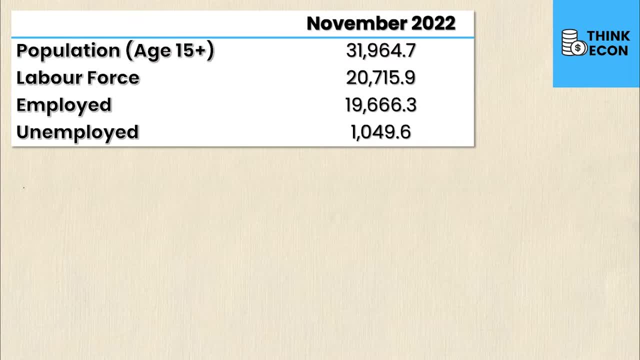 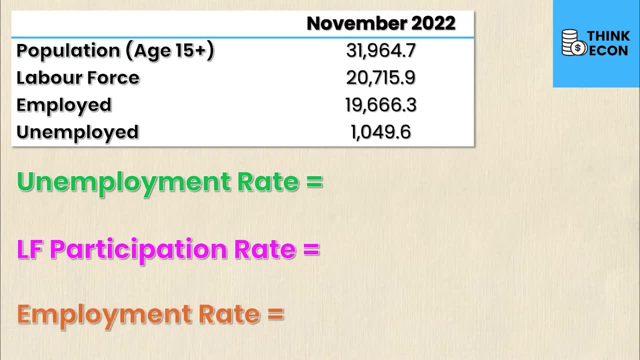 Just thought I'd mention that, in case any of you thought that Canada was just an abnormally small country. So the three rates that we're calculating today are the unemployment rate, the labor force participation rate and the employment rate. Now, these are the three rates.